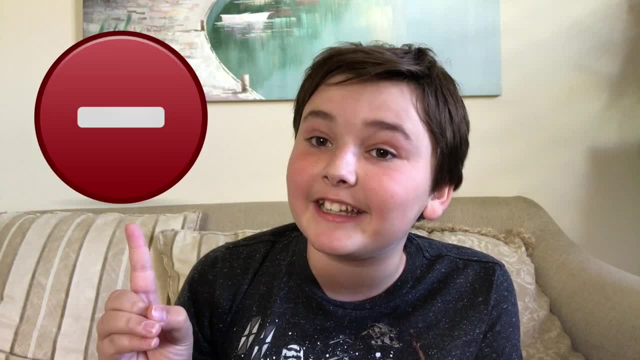 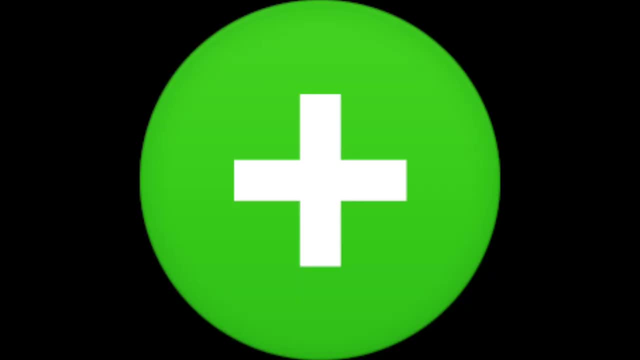 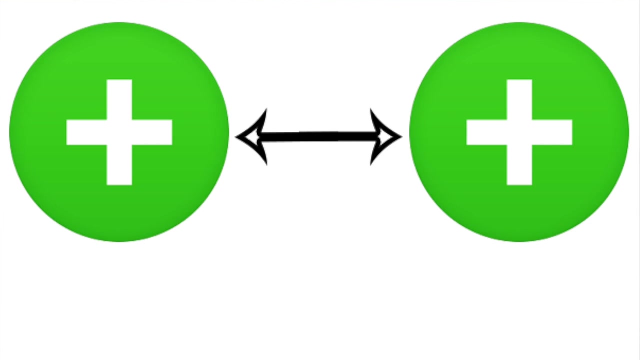 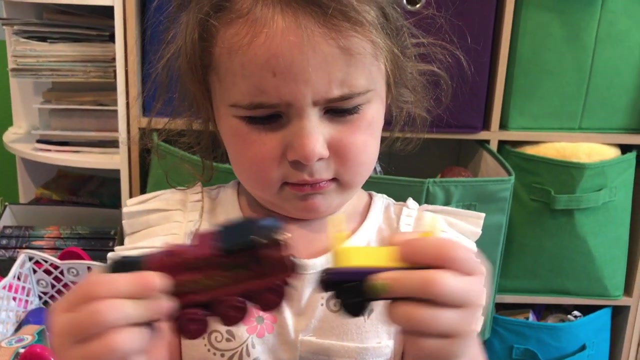 Positive And negative. Each charge likes to be attached with its opposite, So positive likes negative, and the other way around. However, positives move away from other positives, while negatives move away from other negatives. If you've ever played with toy trains that attach to each other, you'll realize that one end is positive and the other is negative. 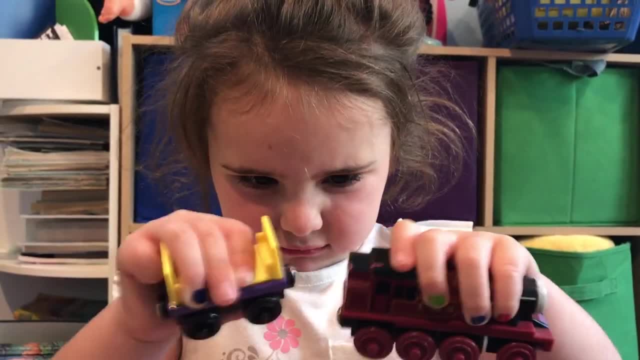 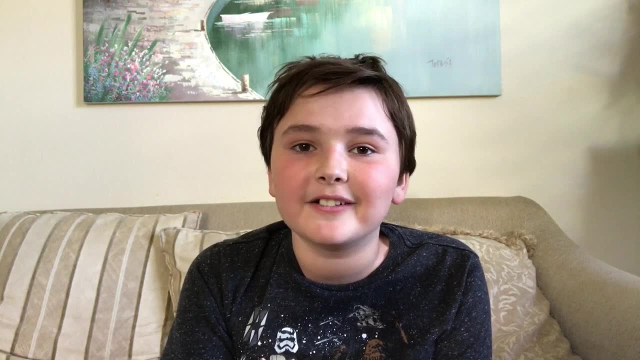 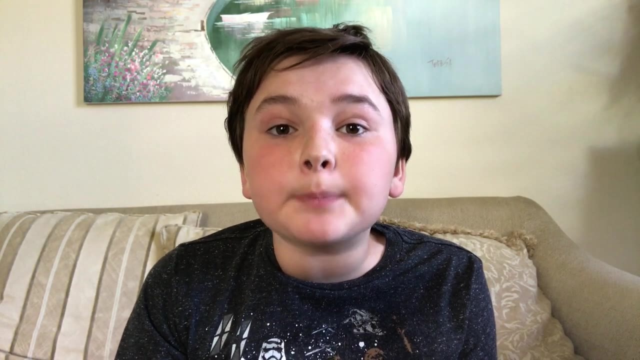 If you try to attach the positives to positives or negatives to negatives, it won't work. Once we realize how electric charges work, we can talk about atoms. I like being talked about. Atoms were once predicted to be the smallest particle of matter. 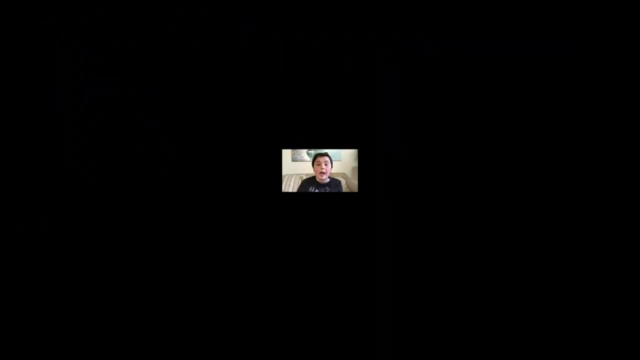 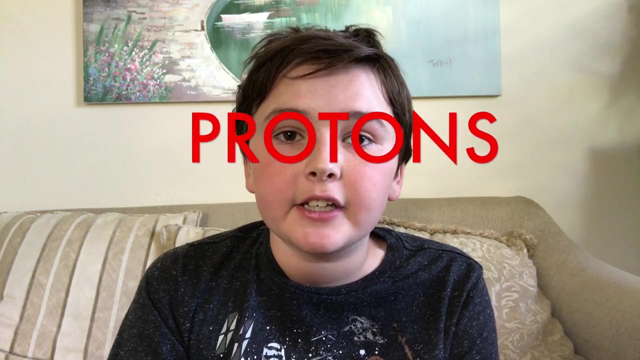 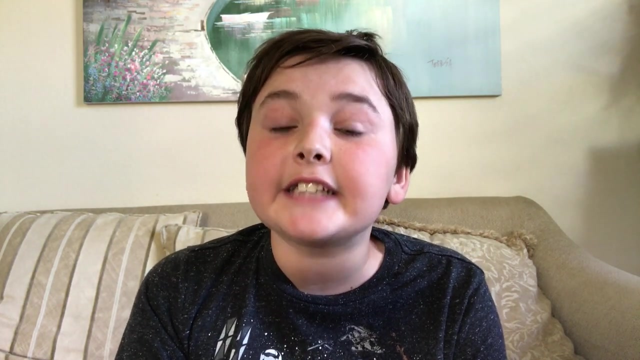 Ugh, Not again. However, scientists have found that atoms are made of three things: Protons, neutrons and electrons. If you ever learned about cells in our body, you'll realize that cells have a nucleus inside them. Atoms also have a nucleus inside them. 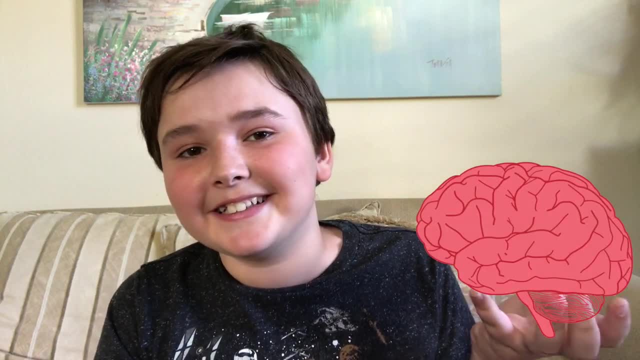 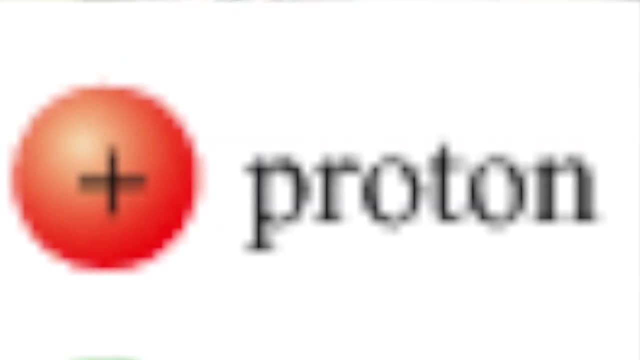 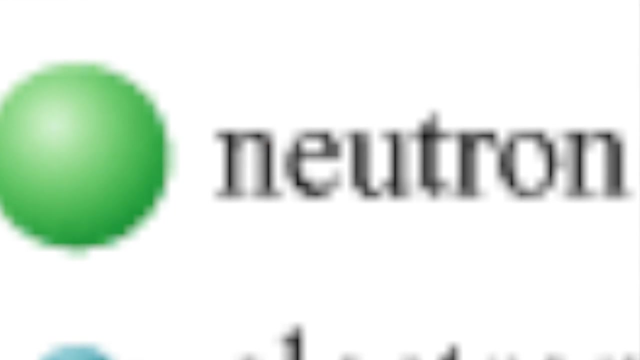 It's kind of like the big brain of the atom. The nucleus is made of neutrons and protons. Protons have a positive charge, while neutrons have no charge. Most of the atoms we know of have all of their protons and neutrons inside the nucleus. 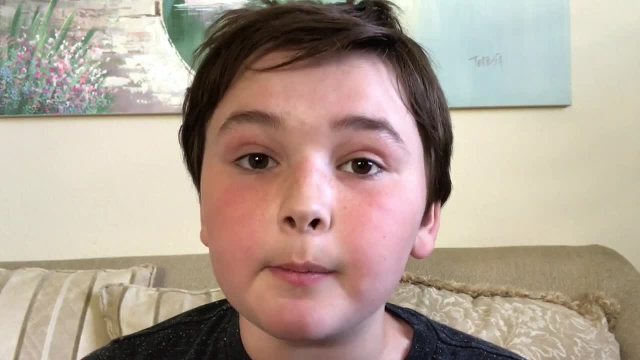 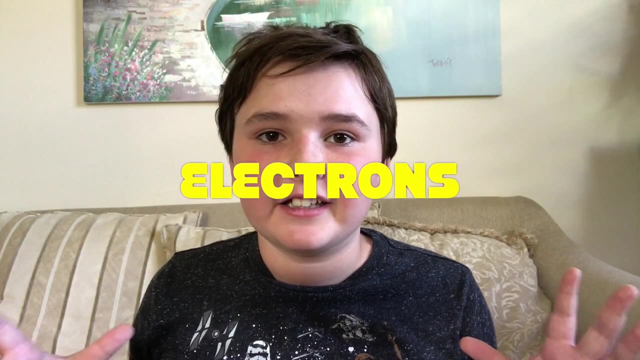 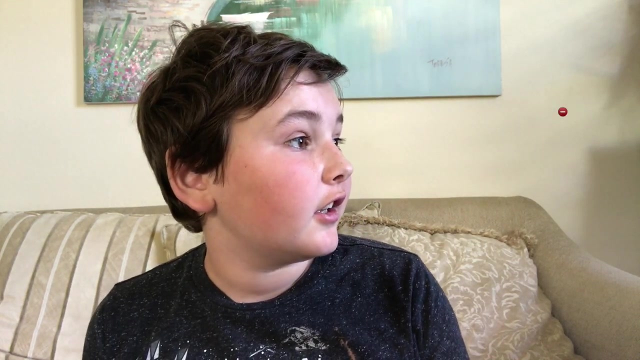 The neutrons have no charge but give the atom more mass and weight. The last part of an atom are the electrons. The electrons are the smallest part of an atom. One tiny little electron is 1,836 times smaller than one of these huge protons. 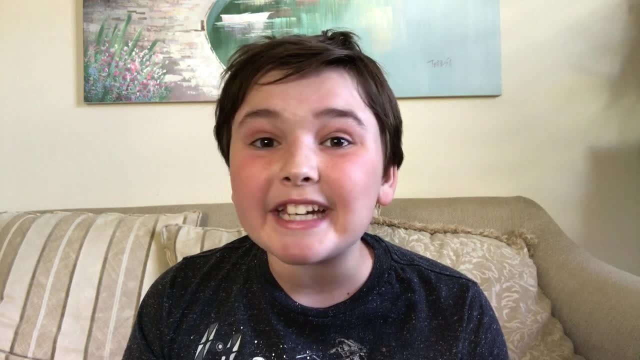 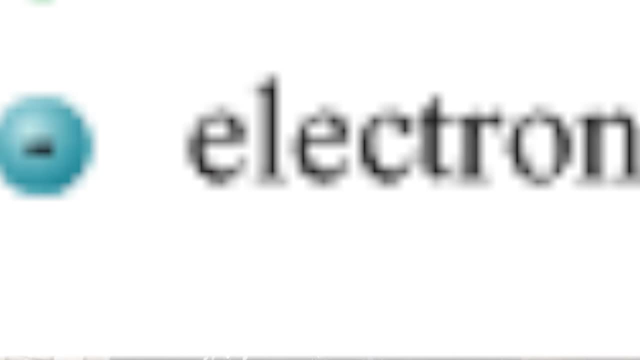 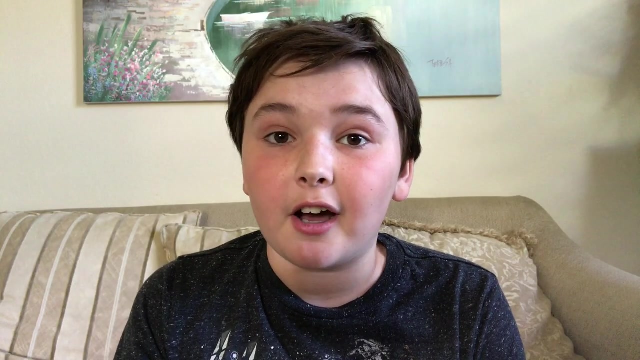 But remember, atoms are so tiny we can't even see them. So imagine how small an electron may be. Electrons have a negative charge. Electrons move around the nucleus in circular motions. They don't attach to protons because- well, remember earlier, they're not a perfect match.